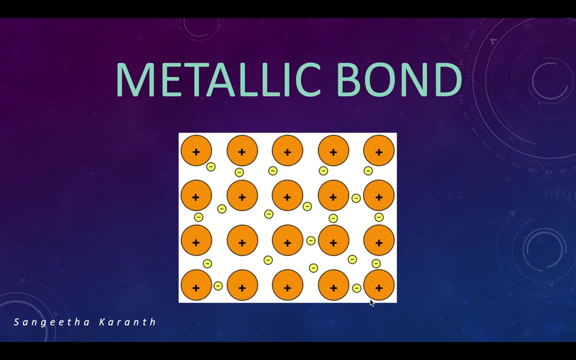 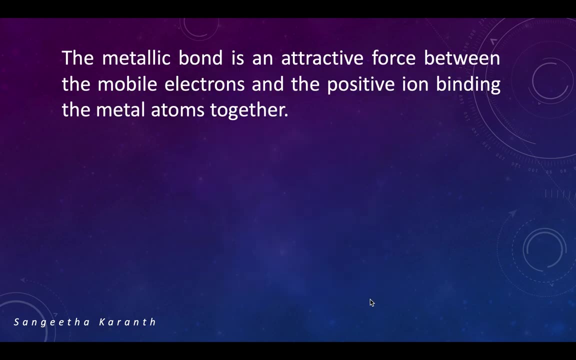 Hello everyone, in this video I'll be explaining about metallic bond and I'll be also discussing about the band theory and electrical properties of metals, semiconductors and insulators. So first coming on to what do you mean by a metallic bond? So metallic bond is nothing but. 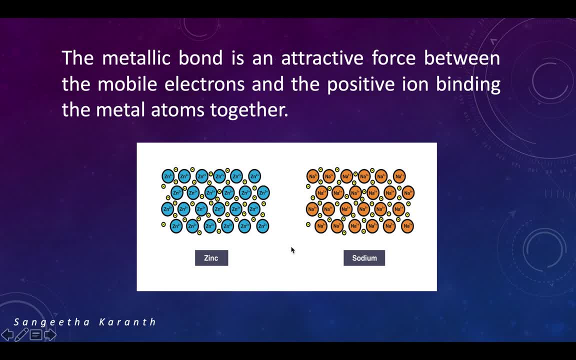 an attractive force which occurs between that of mobile electrons and positively charged metal ions. So here you can see two examples: This is for zinc, These are the zinc ions and these are the mobile electrons. So the attractive force that exists between these mobile electrons, 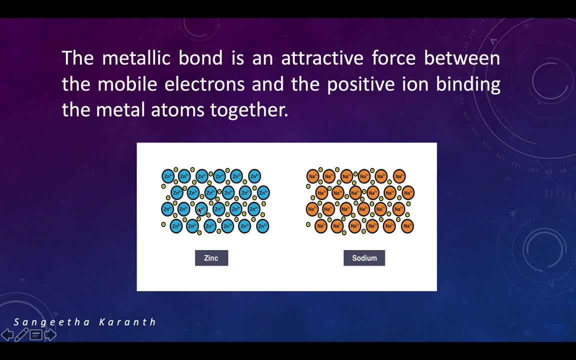 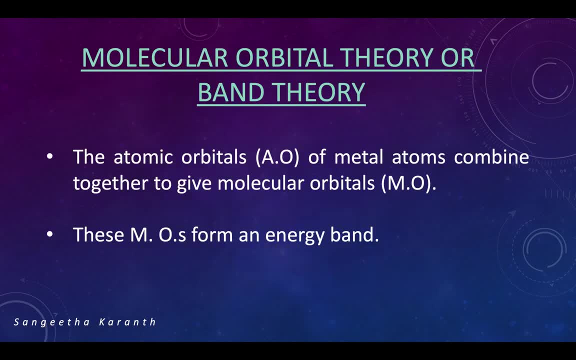 and the zinc ions is nothing but the metallic bond. Same way we can explain it for sodium. So, coming on to what do you mean by a metallic bond? So metallic bond is nothing but a metallic bond. So we know that atomic orbitals will combine together to give molecular orbitals. 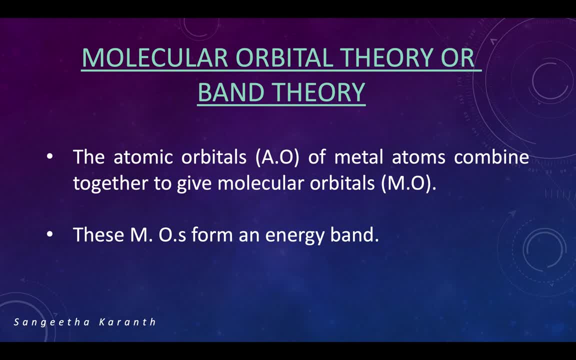 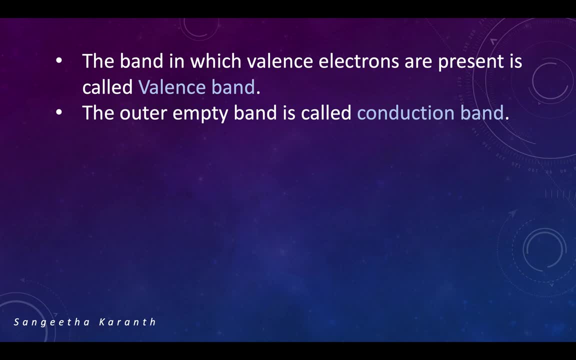 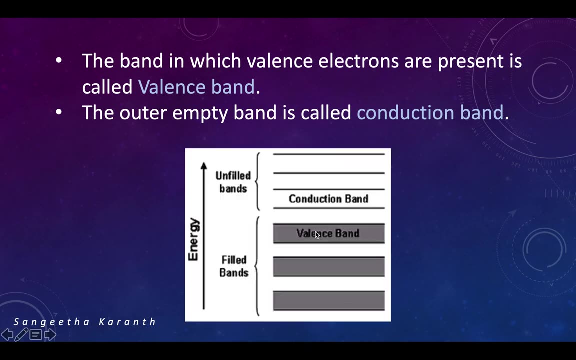 These molecular orbitals form what is known as the energy band, So in metals and related compounds. we first speak about two types of bands, that is, valence band and conduction band. So here we can see it. So this is the valence band and this is the conduction band. 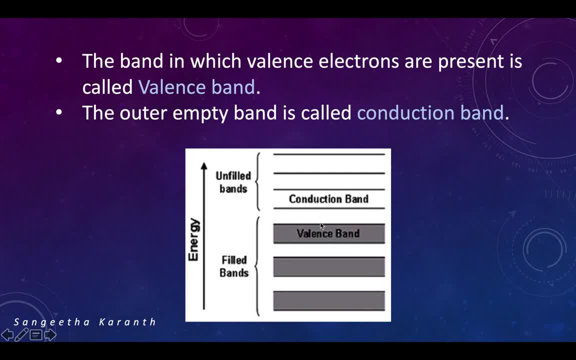 So valence band, as the name indicates, it consists of valence electrons, whereas conduction band, which is the outer band, it is empty. So the valence band consists of valence electrons, whereas the conduction band is empty Only when the electrons from the valence band. 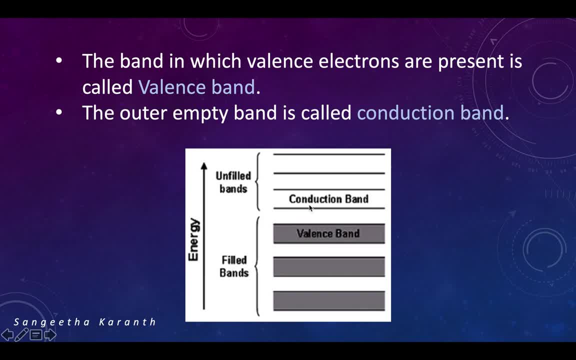 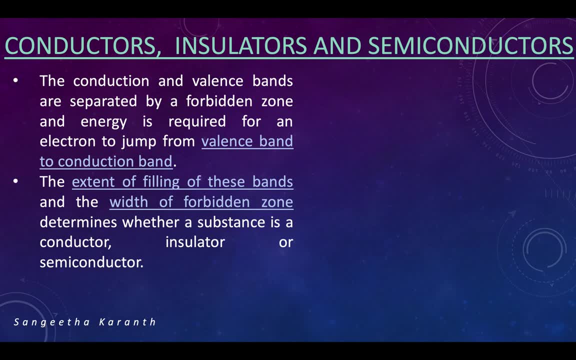 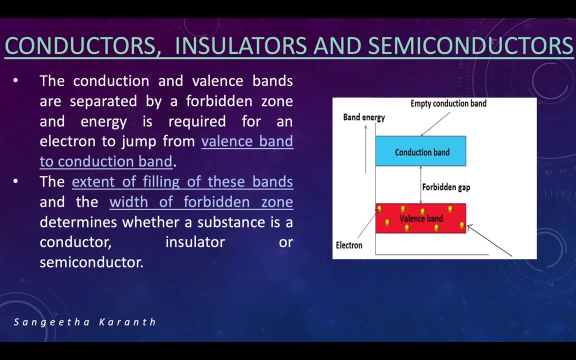 move to the conduction band, then only there will be conduction of electricity. Okay, so now coming on to conduction. So the valence band consists of conductors, insulators and semiconductors. So now we know that the valence band and the conduction band have something called as a 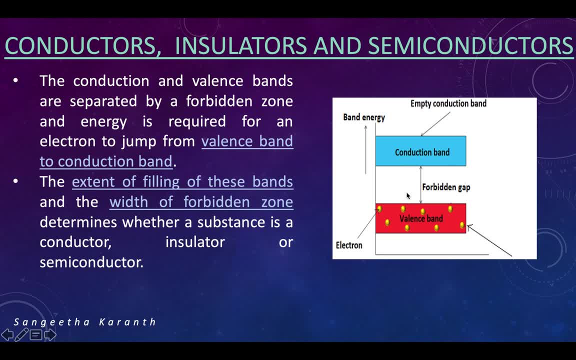 forbidden gap between them. Okay, so this gap is the one which decides whether a particular substance will act as a conductor or whether it will act as an insulator or a semiconductor. Condition is that the electrons have to move from the valence band to the conduction band. 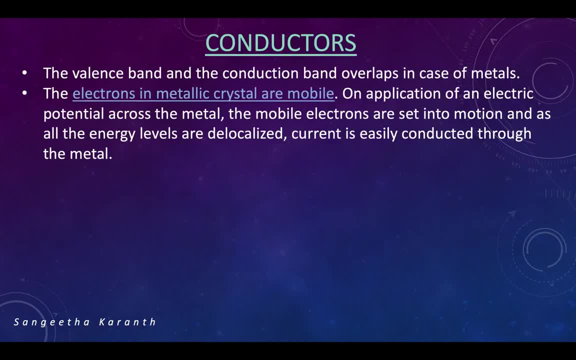 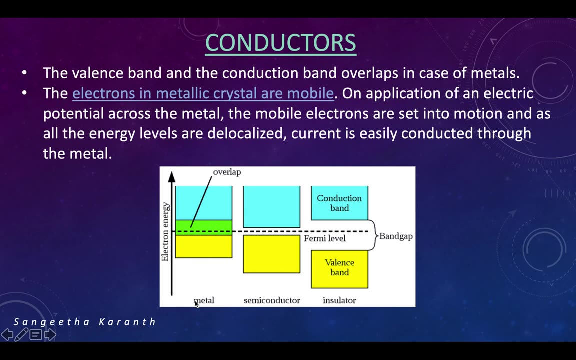 Only then it can act as a conductor. So first coming on to what are conductors and how the valence band and the conduction band are arranged here. So here you can see that here. So this is a comparison of metal semiconductor and insulator. Here you can see conduction band and the valence band are arranged. 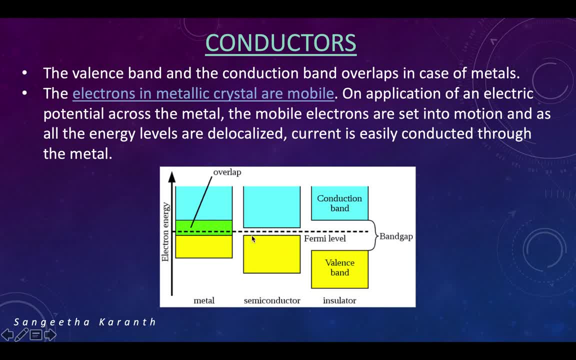 In semiconductor the gap is little less, whereas here the gap between valence band and conduction band is very high. Okay, so here, since there is an overlap between the conduction band and valence band, the electrons can easily move from valence band to the conduction band when an electric 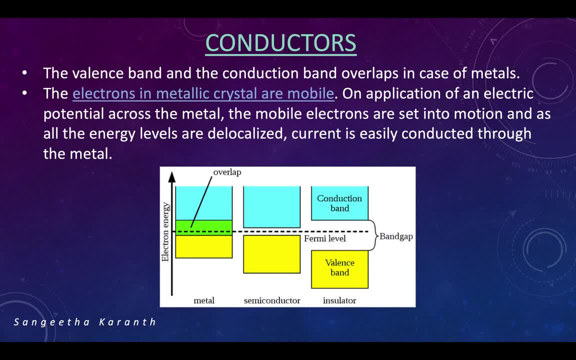 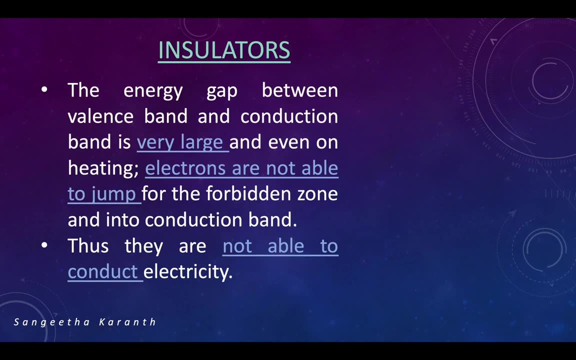 potential is applied. So here this type of substances, where there is an overlap between the two bands, can easily act as conductors, So that the current is easily conducted through these materials. Next, coming on to insulators. Here you already know that in the previous slide I have 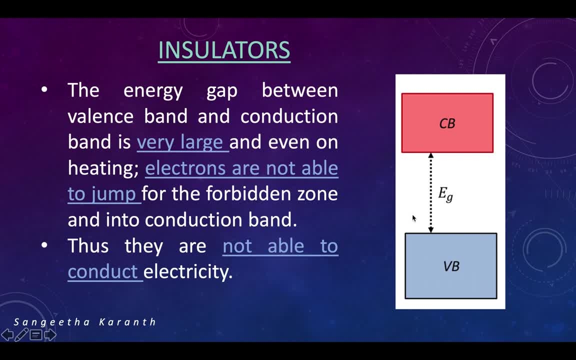 shown it. So valence band and conduction band: the gap between them is very high. Here you can see this. the energy gap is very high, So much energy is required for the electrons to move from the valence band to the conductor. So here you can see that the electrons can easily act as conductors. 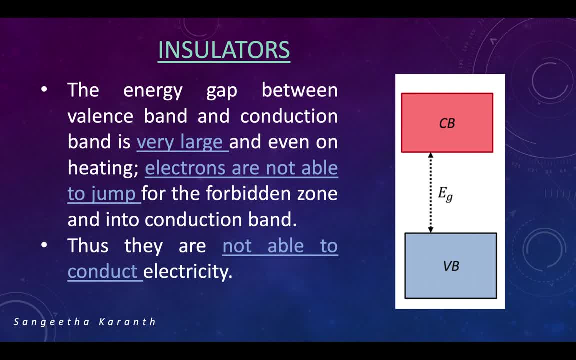 conduction band. So what happens here is very large amount of energy is required for the electrons to move from valence to conduction band. So here the movement of electrons is forbidden. Okay, so because of this, these type of materials are not able to conduct electricity Coming on to. 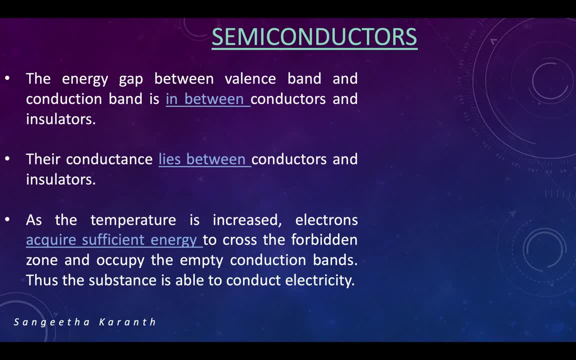 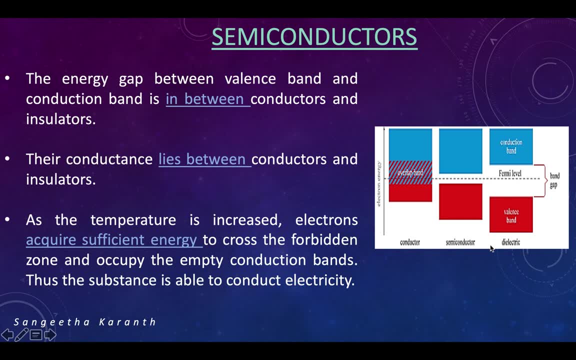 semiconductors. So you have already seen the comparison. So here you have seen, in conductors there is an overlapping of the two bands. In the insulators the gap is very high, Whereas in semiconductor the gap is intermediate between these two. Here we know that in conductors they can easily conduct electricity, Whereas insulators. 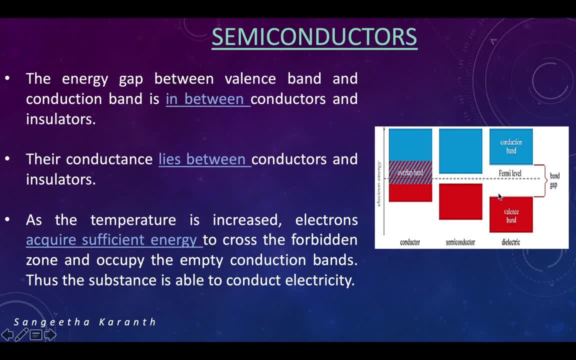 they cannot conduct electricity because movement of electron is highly forbidden, Whereas in semiconductors the gap is in between these both. So we can say that if energy is given to the electrons, then the electrons can easily jump from valence band to the conduction band. So here what is? 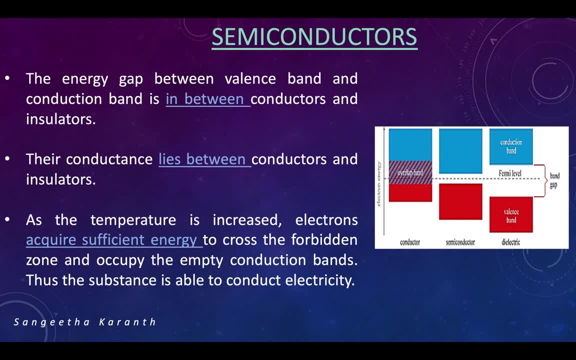 the energy given to the electrons. So mainly energy is given in the form of increase in temperature. So as the temperature is increased the electrons will gain energy and move from the valence band to the conduction band. So here the movement is quite easier when compared to the insulators, So semiconductors- 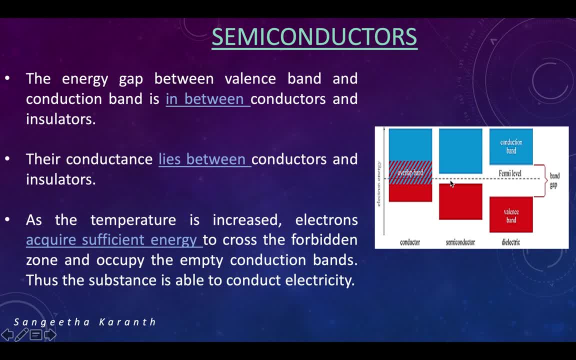 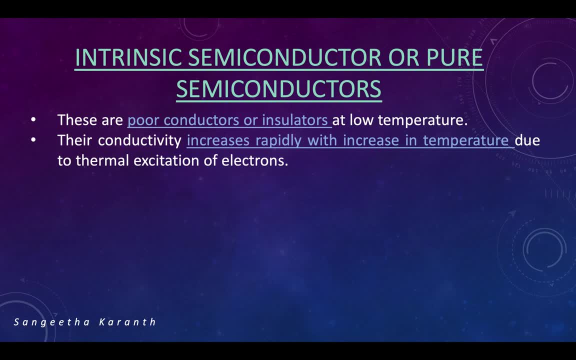 can also conduct electricity under specific conditions. So here in semiconductors again we have two types: intrinsic semiconductors and extrinsic semiconductors. First we will deal with intrinsic semiconductor. Intrinsic semiconductor is also known as pure semiconductor. So here 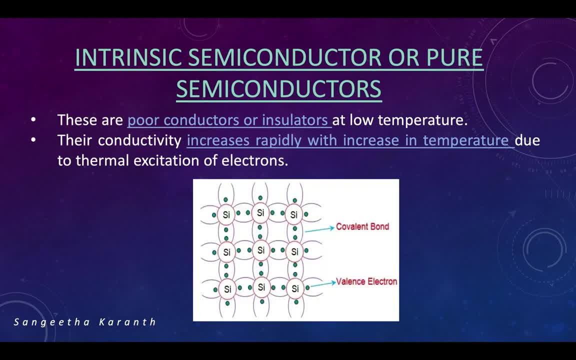 we can take the example of silicon. So here we are only speaking about the silicon atoms, which are joined together by means of covalent bonds. So these electrons are the ones which are involved in bonding and these are the terminal electrons. okay, or we can also call them as valence electrons. 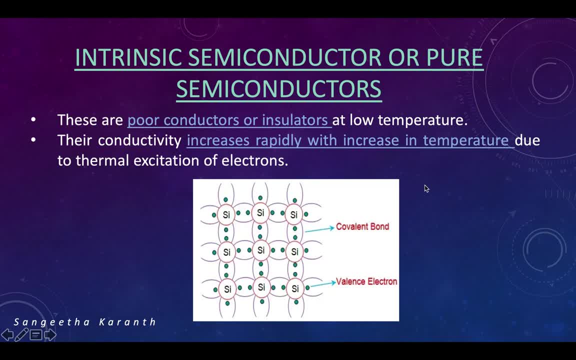 okay, So here also silicon is an example for a semiconductor. So we know that the energy gap between the conduction and the valence band is less, and hence silicon can act as a semiconductor. but here we are not using any other atom, So silicon is an atom other than silicon. so it is also called as pure semiconductor, and it is also. 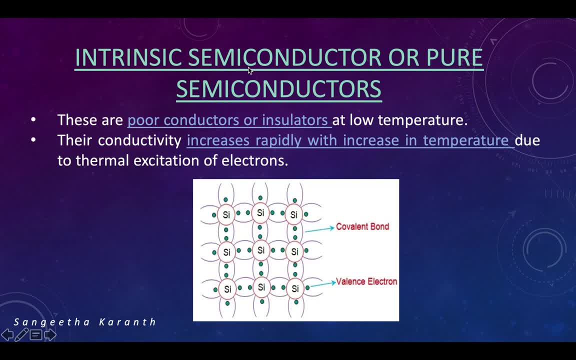 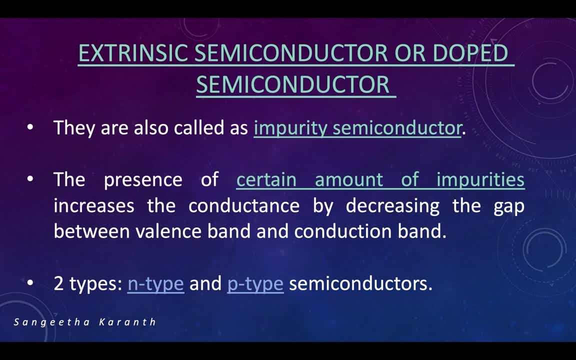 referred to as intrinsic semiconductor. So what is extrinsic semiconductor? If intrinsic is pure semiconductor, then extrinsic is nothing but doped semiconductor. Now, what is doping? Doping is nothing but adding an impurity. okay, So these are also called as impurity semiconductors. So here: 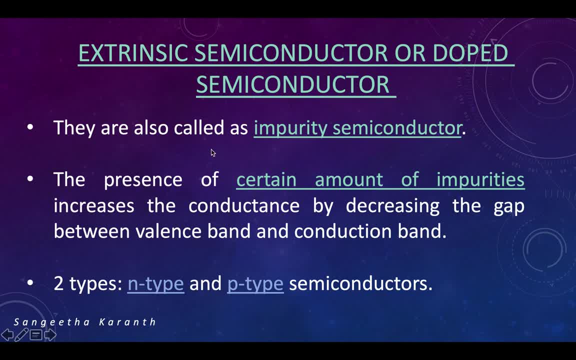 in such type of semiconductor we have two types of semiconductors. So here in such type of semiconductor we add a certain amount of impurities. so if these impurities are added to these intrinsic semiconductor, then the conductance will be increased. So two types of impurities can be. 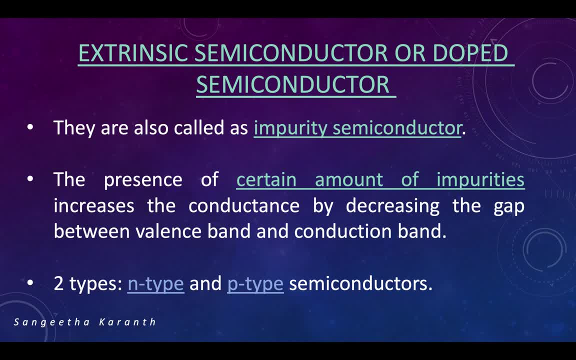 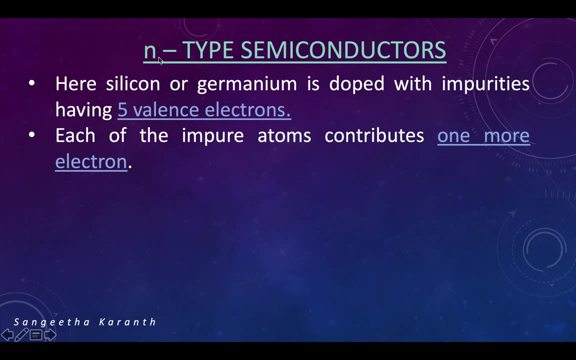 added. If such impurities are added, we get two types of semiconductors. The semiconductors are named as n- type and p-type semiconductors. So first let us see what you mean by n type semiconductor. here the term n that indicates it is negative. So negative is nothing, but there should be more. 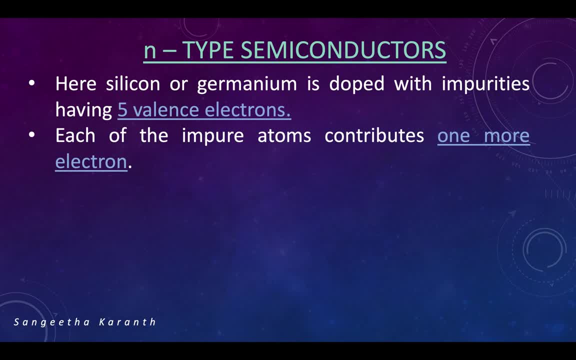 of electrons. We know that silicon or germanium have only four electrons in the valence shell. Suppose you add an impurity with five electrons in the valence shell, then we know that the number of electrons will be one extra. So suppose we add a certain amount of impurity. atoms with five. 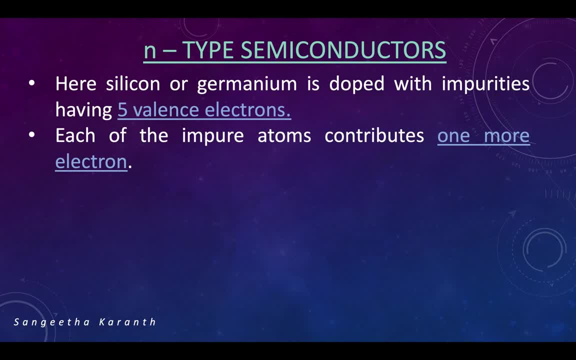 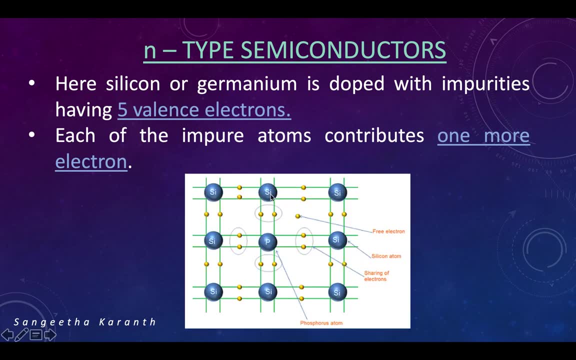 valence electrons, then obviously there will be more number of electrons than the pure silicon or germanium. So here we can see the example. So silicon, all these atoms are silicon, where one impurity of phosphorus is added. Phosphorus as, as you all know, it has five valence electrons. 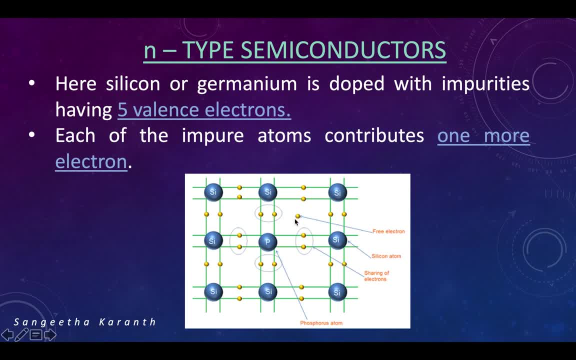 and hence, here you can see, one electron is extra. So this extra electron, okay, which is formed from one impurity atom. Similarly, we add many impurity atoms, So there are many number of extra electrons. So these extra electrons are responsible for conductance. okay, So these extra electrons. 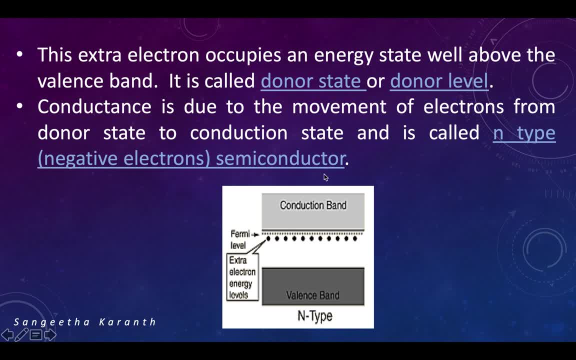 form a particular level which you can see here. okay, So this level, it forms this extra level which is also called as donor state or donor level. So the movement of electrons take place from this donor state to the donor state. So this is the donor state, So the movement of electrons. 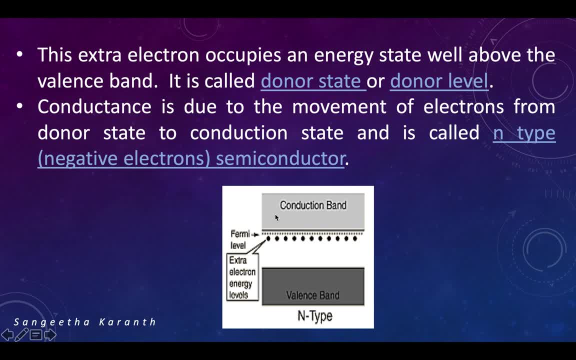 takes place from the donor level to the conduction band, which is much easier. So here such type of semiconductor semiconductors are called as n-type semiconductors. N is again referred to as negative type, which is due to the extra electrons of the impurity that is added. So what is p-type? 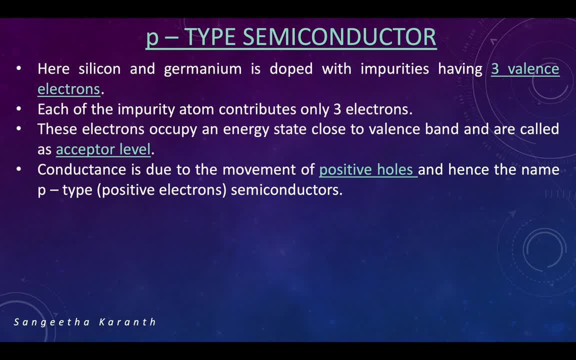 semiconductor N-type refers to negative, so P should refer to positive. So if it is positive, that means the number of electrons is less than or equal to negative. So if it is positive, that means the number of electrons is less than required. So we know that again, silicon and germanium have four electrons in the valence shell. 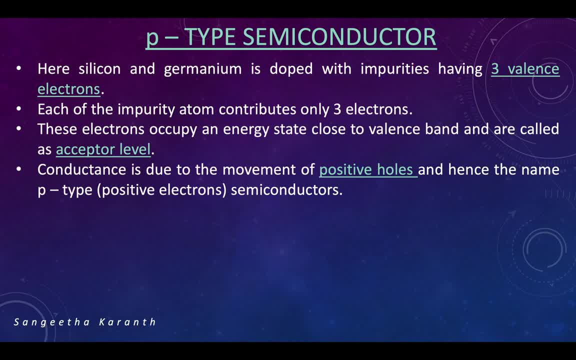 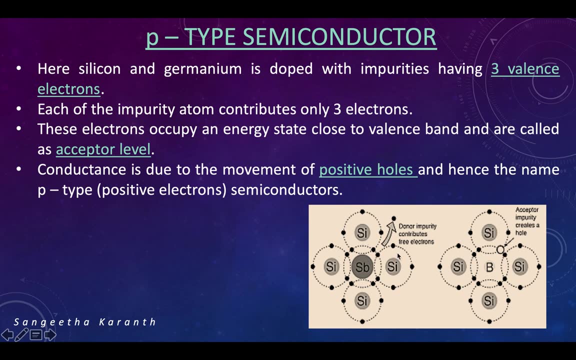 So suppose you add an impurity with one electron less, that is, with only three valence electrons, then there will be a deficiency of electron. So this will create holes in those places. So you can see, here all these are silicon. So here these are the impurities that are added. So here, if you add, 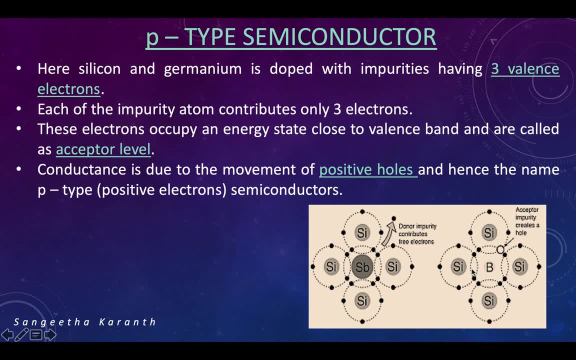 boron in this place as an impurity. boron has only three electrons in its valence shell, So it creates a hole, or we can say it creates a vacancy where one electron is less. So this hole, so we call it as positive because it is due to deficiency of electron. So these positive holes make a particular 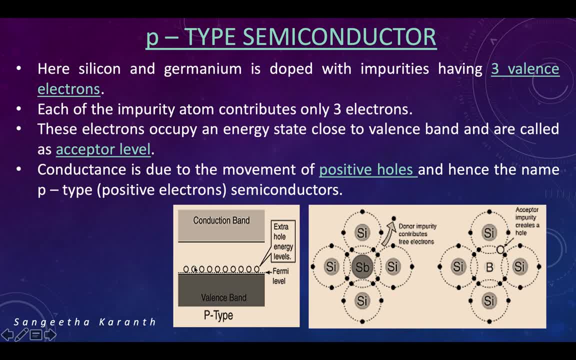 level here okay, and thus the movement of holes will result in the conductance in this type of semiconductor. So we know that the semiconductors are of two types. One is intrinsic, which is pure, that is only silicon or only germanium. Next is extrinsic, which is caused. 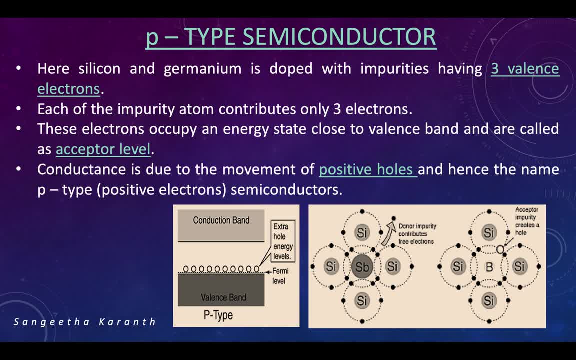 due to doping. So doping can be brought about in two different types: by adding an impurity with more number of electrons or adding an impurity with less number of electrons. If we add an impurity with more number of electrons, that is, with five valence electrons, then we get an. 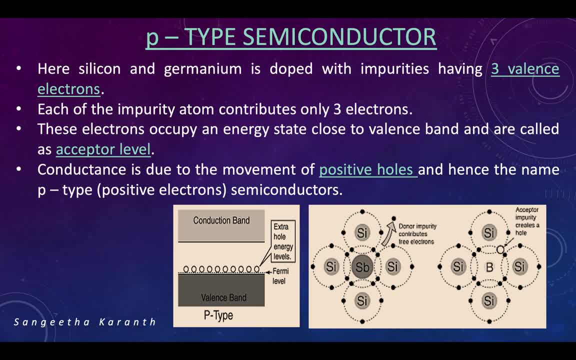 n-type semiconductor. Same way, if we add an impurity with less, that is with three valence electrons, we get a p-type of semiconductor. So both this type of semiconductors, that is p and n-type, will have more conductance when compared to that of intrinsic semiconductors. So in this 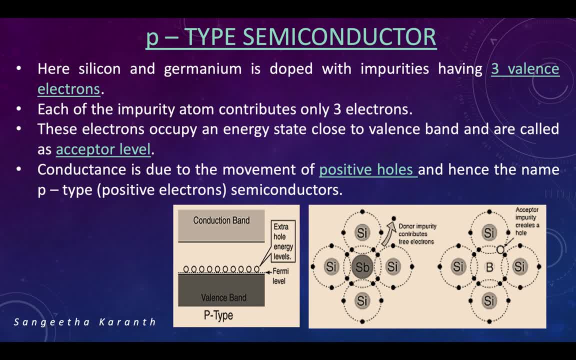 video I have covered what do you mean by metallic bond and what are the different types of semiconductors. So in this video I have covered what do you mean by metallic bond and what are the different types of substances based on the gap between valence band and.